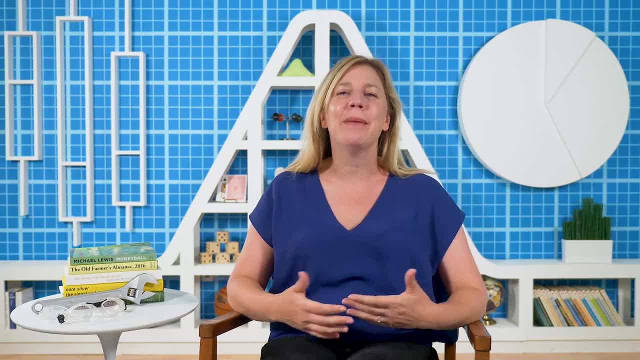 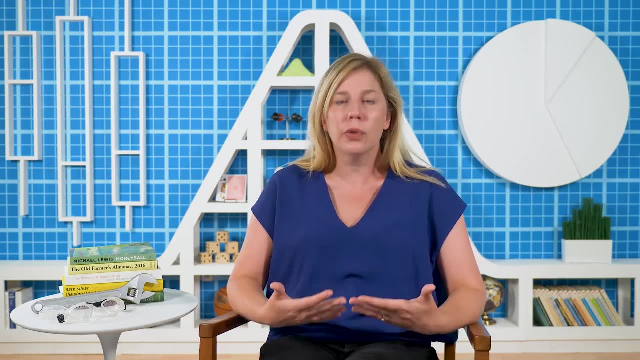 Hi, I'm Adriene Hill and welcome back to Crash Course Statistics. Sometimes random variation can make it tricky to tell when there are true differences or if it's just random, Like whether a sample difference of $20 a month represents a real difference between 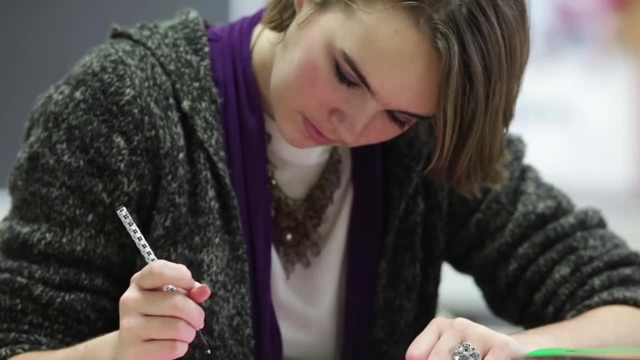 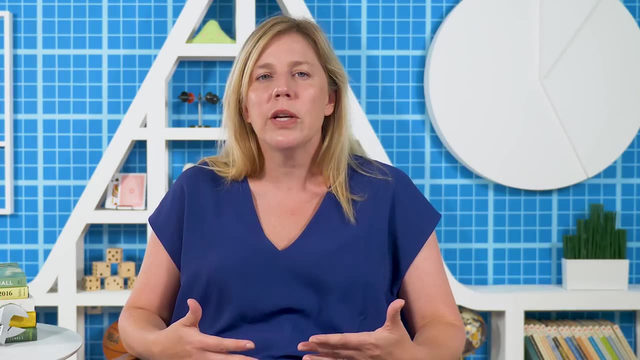 the average rates of two car insurance companies, or whether a one-point increase in your AP stats grade for every hour you study represents a real relationship between the two. These situations seem pretty different, but when we get down to it they share a similar. 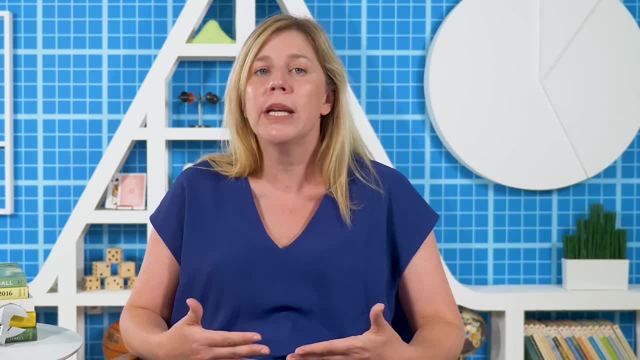 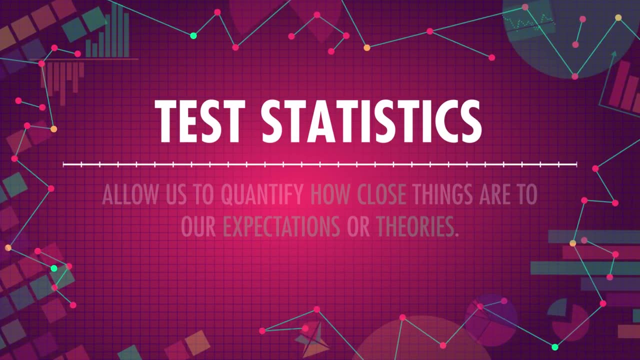 pattern. There's actually one idea which, with a few tweaks, can help us answer all of our is it random or is it real questions. That's what test statistics do. Test statistics allow us to quantify how close things are to our expectations or theories. 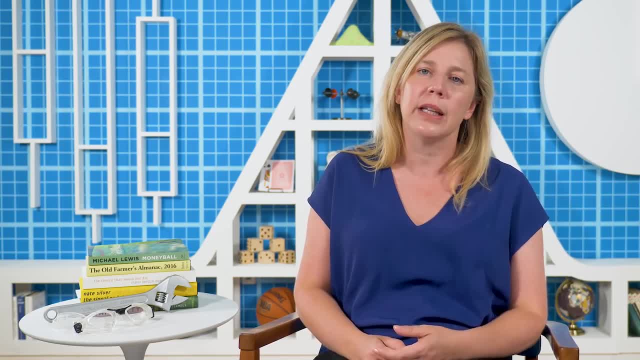 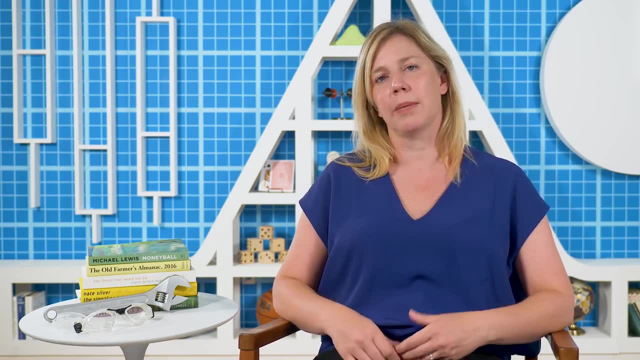 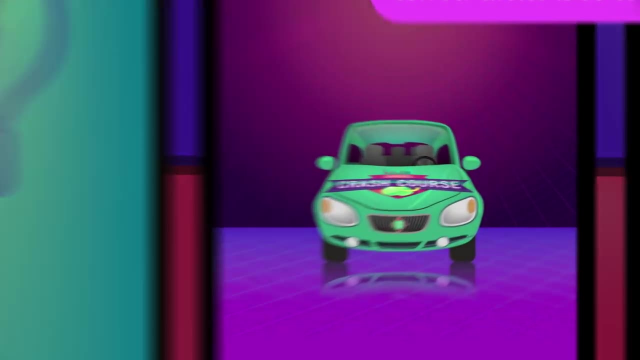 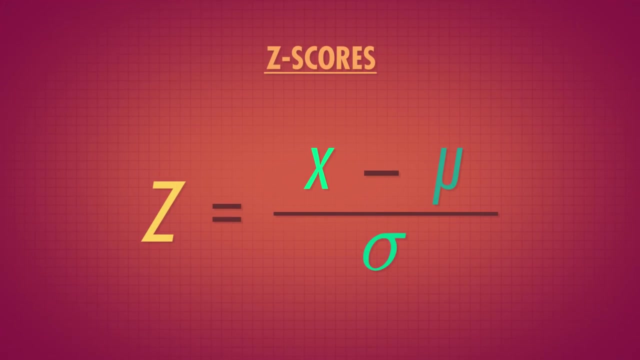 – something that's not always easy for us to do, based on gut feelings And test statistics. allow us to add a little more mathematical rigor to the process, so that we can make decisions about these questions. In previous episodes, z-scores helped us understand the idea that differences are relative. 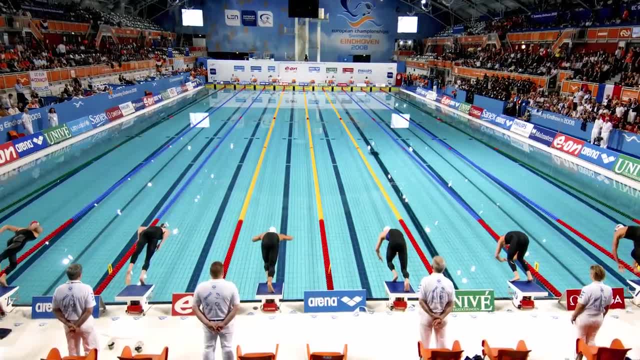 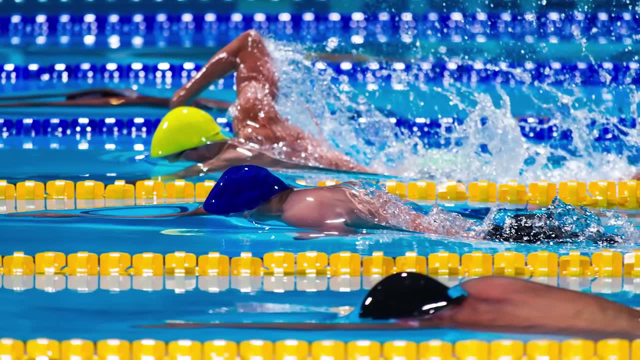 A difference of one second is meaningful if, say, you're looking at the differences in the average time, it takes two groups of elite Olympic athletes to complete a 100-meter freestyle swim. It's less meaningful when you're looking at the differences in the average time it. 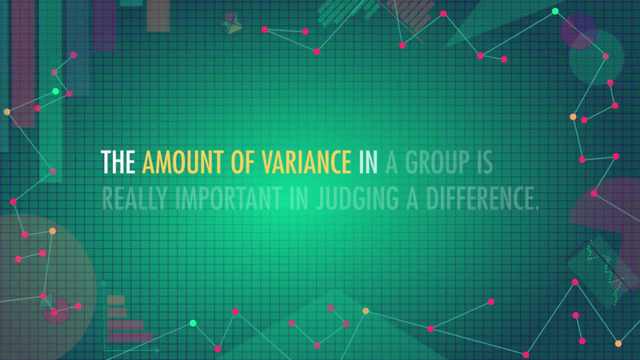 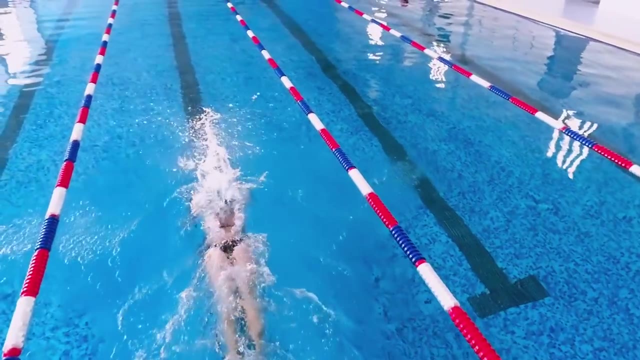 takes two groups of recreational swimmers. The amount of variance in a group is really important in judging a difference. Elite Olympic athletes vary only a little bit. Their 100-meter times are relatively close together and a tenth of a second can mean the difference between a gold and a bronze medal. 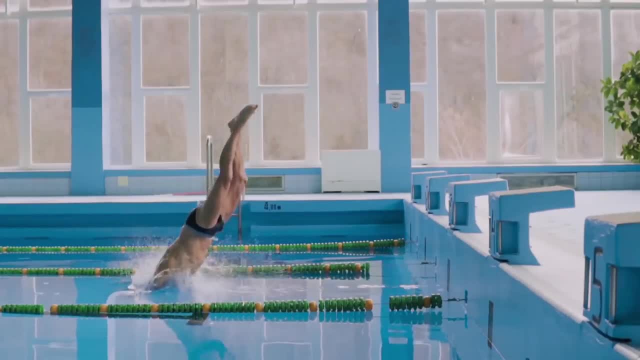 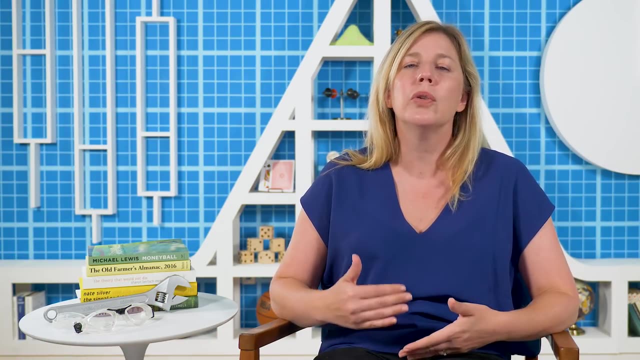 Whereas non-professionals have more variation. The fastest swimmers could finish a whole minute or more before the slower swimmers. A difference of one second isn't a big deal. It's more meaningful between two groups of recreational swimmers, because the difference 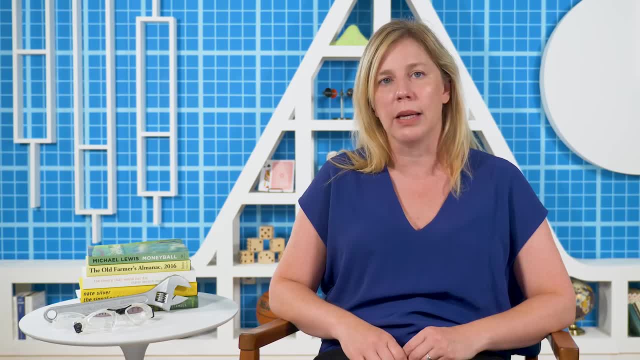 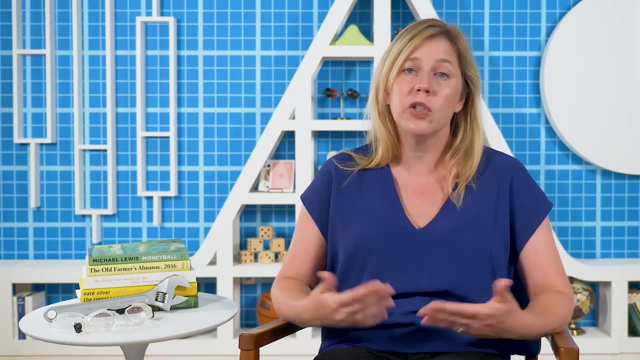 is small compared to the natural variation we'd expect to see. Two groups of casual swimmers may differ by 10 or more seconds, even if their true underlying times were the same, just because of random variation. That's why test statistics look at the difference between data and what we'd expect to see. 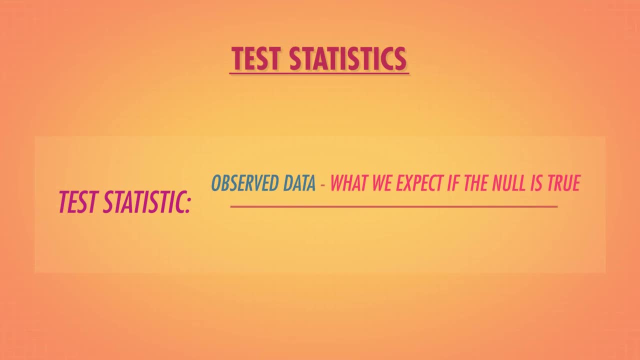 if the null hypothesis is true. But they also include some very important context: A measure of the average variation we'd expect to see, Like how much novice or pro swimmers would be able to do it. Test statistics help us quantify whether data fits our null hypothesis well. 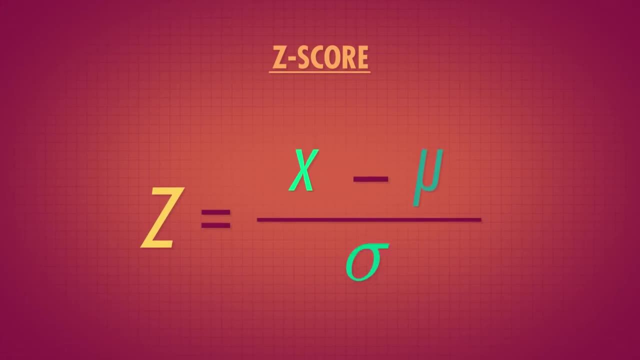 A z-score is a test statistic. Let's look at a simple example. Say your IQ is 130.. You're so smart And the population mean is 100.. On average, we expect someone to be about 15 points from the mean. 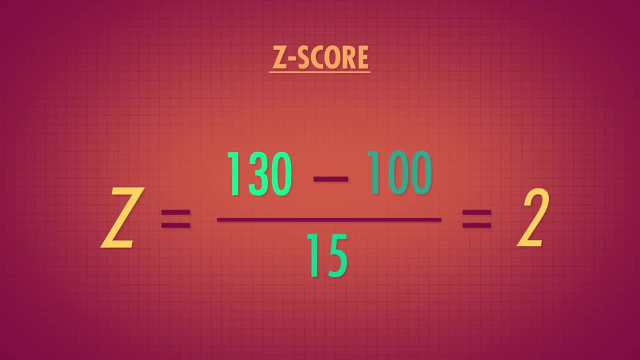 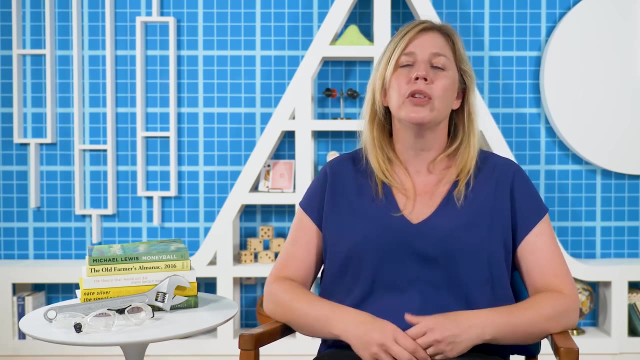 So the difference we observed- 30, is twice the amount we'd expect to see. on average, Your z-score would be 2. And you can z-score any normal distribution, Like a population distribution, But also a sampling distribution, which is the distribution of all possible group means. 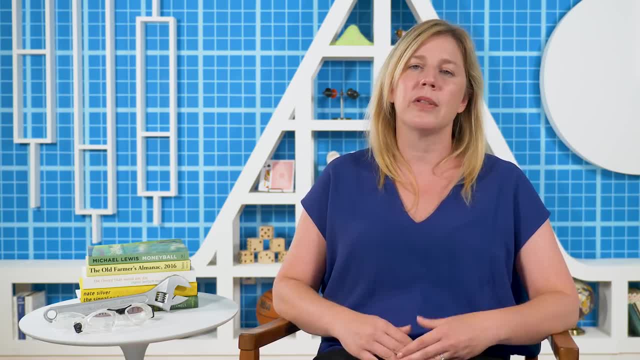 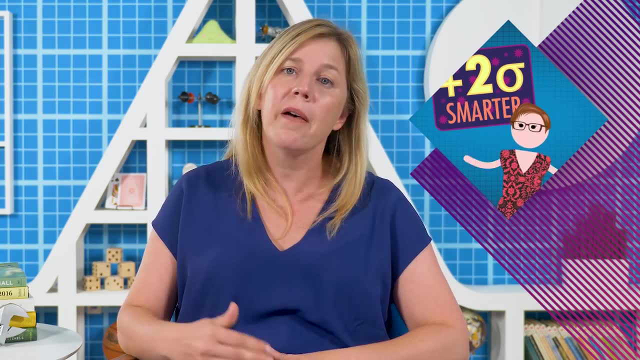 for a certain sample size. You might remember we first learned about sampling distribution in episode 19.. We often have questions about groups of people Finding out that your two standard deviations above the mean for IQ is pretty ego boosting but it's not really going to help further science. 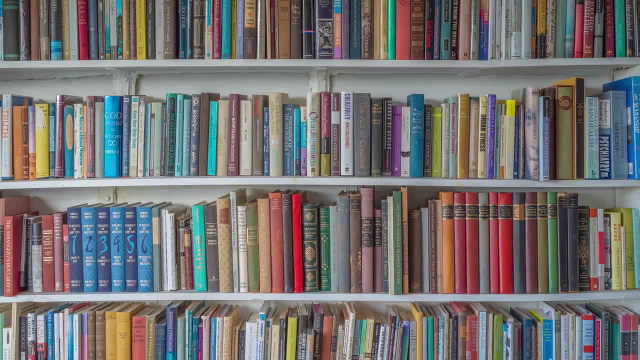 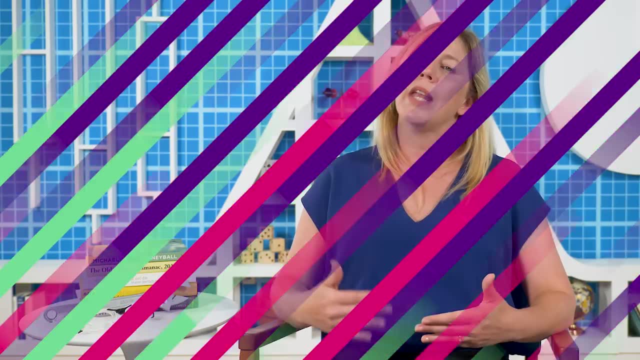 We could look at whether children with more than 100 books in their room have higher than average IQs. Let's say we take a random sample of 25 kids With over 100 books. Then we measure their IQs. The average IQ is 110.. 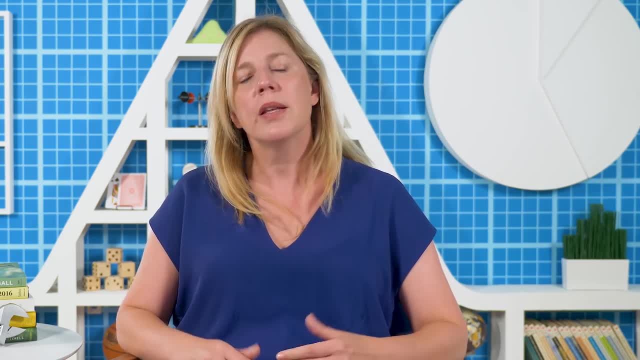 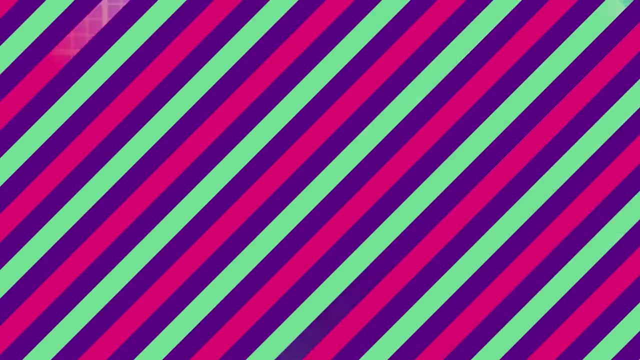 We can calculate a z-score for our particular group mean. The steps are exactly the same. we're just now looking at the sampling distribution of sample means rather than the population distribution. Instead of taking an individual score and subtracting the population mean, we take a 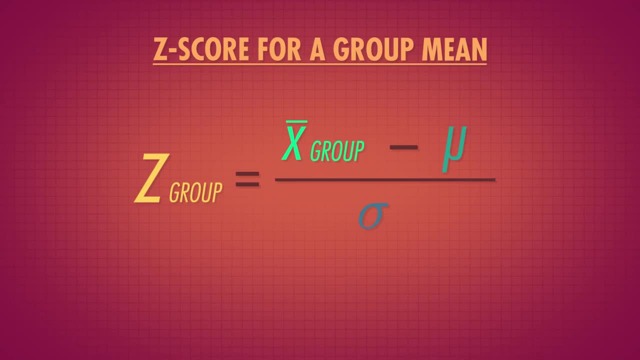 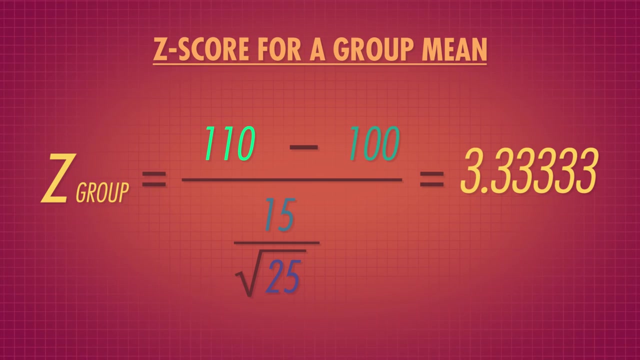 group mean and subtract the mean of our sampling distribution under the null hypothesis. Then we divide by the standard error, Which is the standard deviation. The z-score, also called the z-statistic, tells us how many standard errors away from the sampling distribution mean. our group mean is. 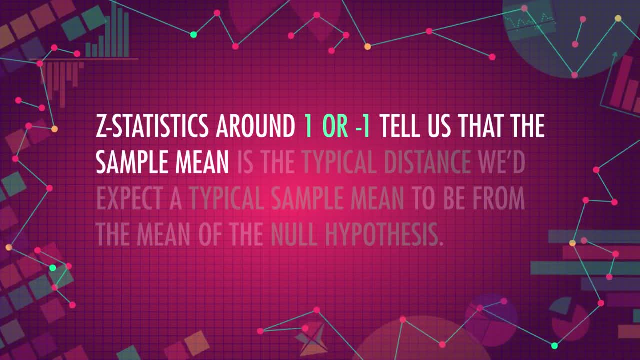 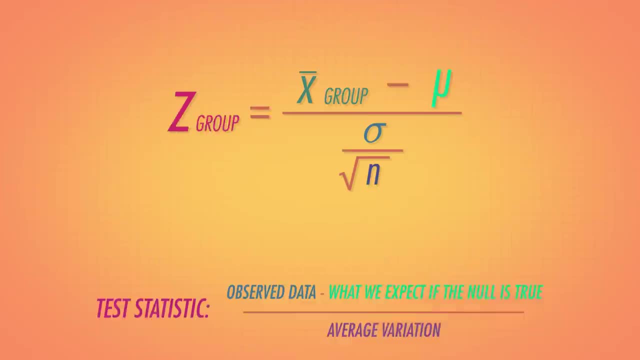 Z-statistics around 1 or negative 1 tell us that the sample mean is the typical distance. we'd expect a typical sample mean to be from the mean of the null hypothesis. Z-statistics that are a lot bigger in magnitude than 1 or negative 1 mean that this sample 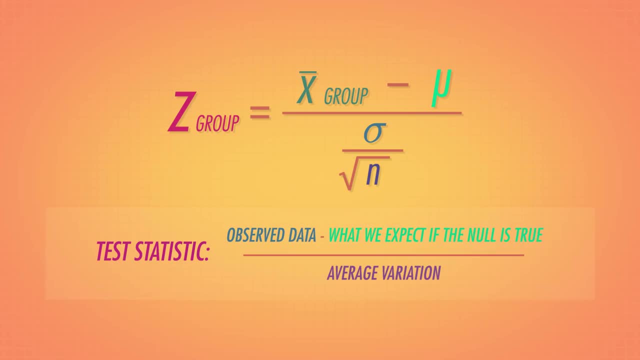 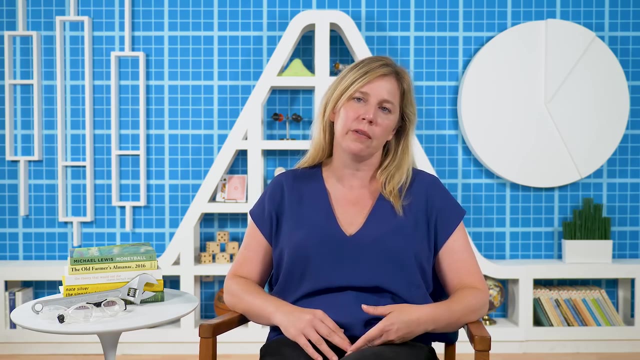 mean is more extreme, Which matches the general form of a test statistic. The p-value will tell us how rare or extreme our data is, so that we can figure out whether we think there's an effect, like whether children with more than 100 books in their 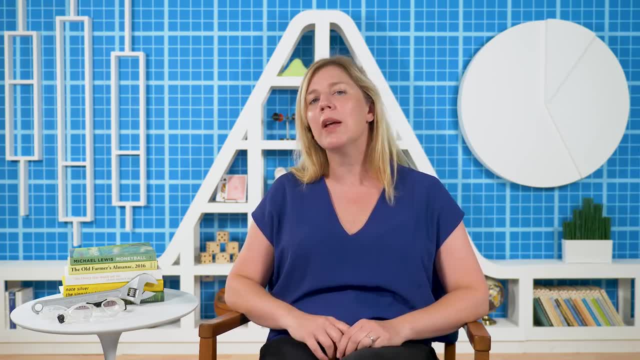 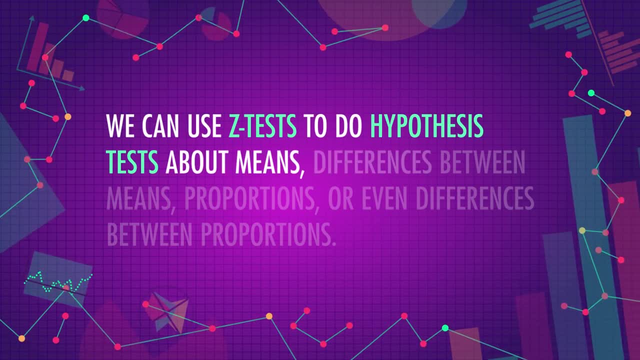 home have a higher than average IQ. Historically we've done this with tables, but most statistical programs, even excel, can calculate this. We can use z-tests to do hypothesis tests about means, differences between means, proportions or even differences between proportions. 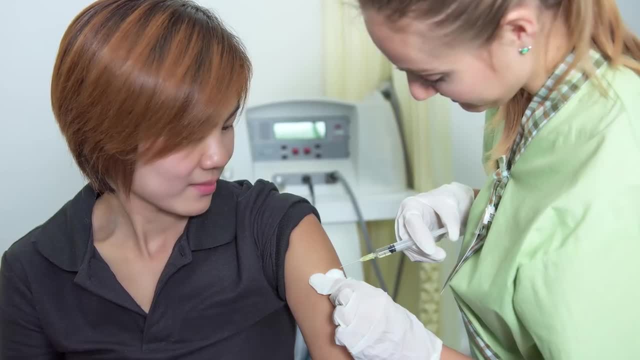 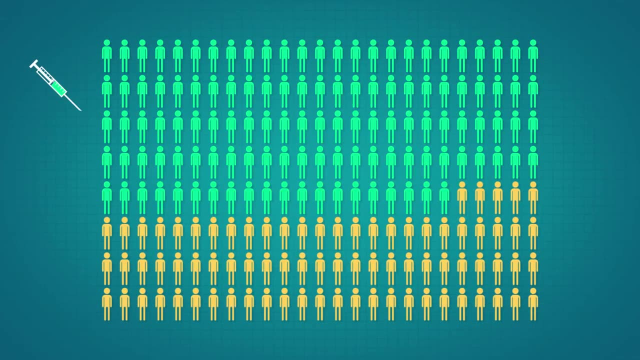 A researcher may want to know whether people in a certain region who got this year's flu-vaccine were less likely to get the flu. They randomly sampled 1,000 people and found that 600 people got the flu vaccine and 400. 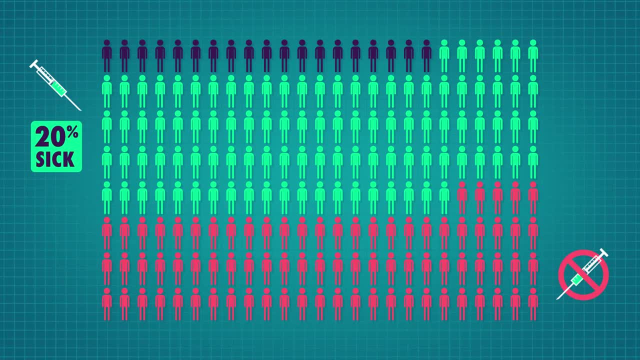 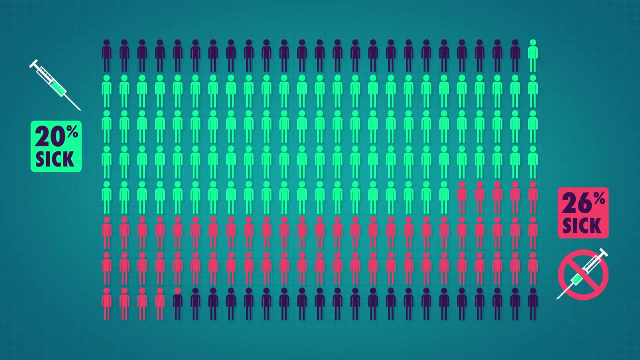 didn't. Out of the 600 people who got the vaccine, 20% still got the flu. Out of the 400 people who did not get the vaccine, 26% got the flu. It seems like you're more likely to get the flu if you didn't get a flu shot. 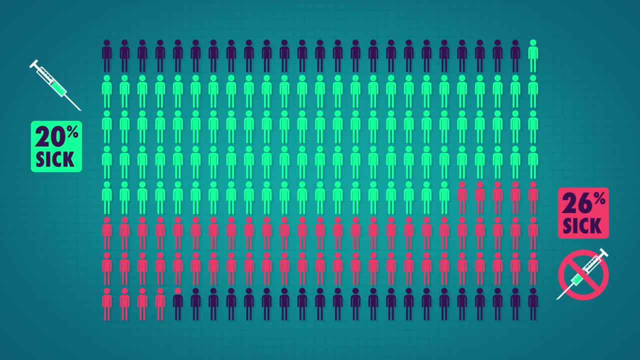 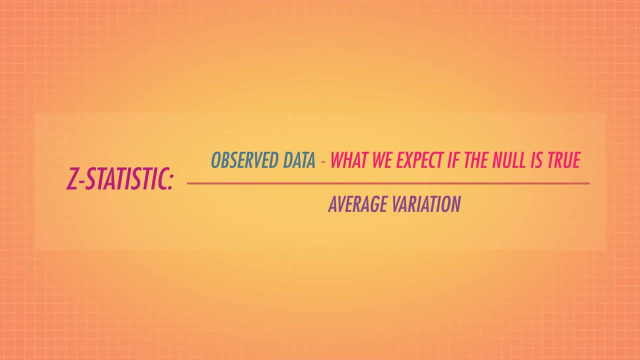 But we're not sure if this difference is pretty small compared to random variation or pretty large. To calculate our z-statistic for this question, we find that the number of people who got the flu first has to remember our general form. There's a 6% difference between the proportion of the vaccinated and unvaccinated groups. 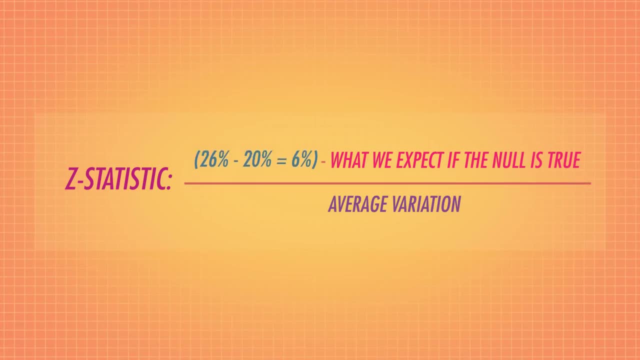 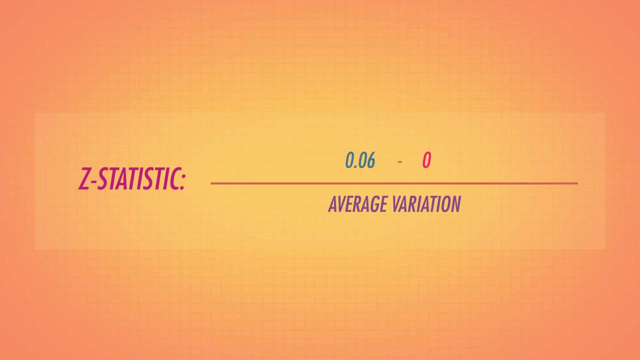 and we want to know how different 6% is from 0%. A difference of 0% would mean there's no difference between flu rates between the two groups. So our observed difference is 6 minus 0% or 6%. For this question, the average variation of what percent of people get the flu is the. 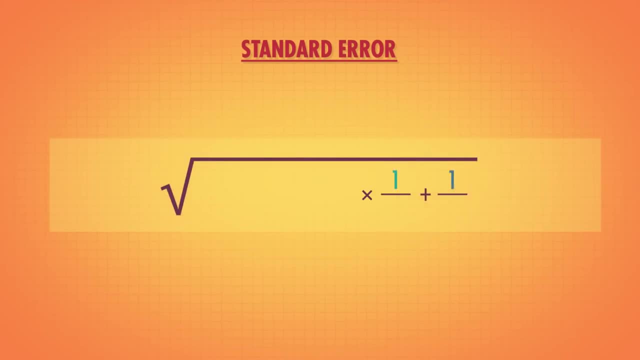 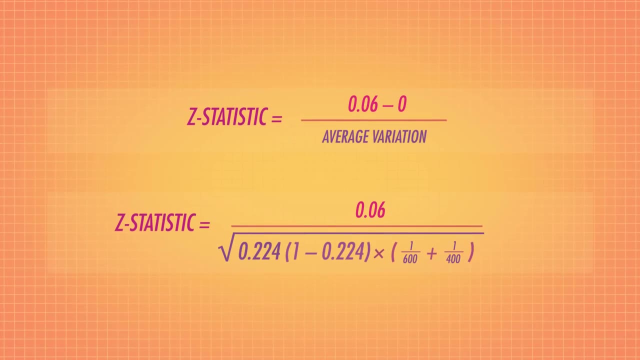 standard error from our sampling distribution. We calculate it using the average proportion of people who got the flu and didn't get the flu. If our observed difference of 6% is large compared to the standard error, which is the amount of variation we expect by chance, we consider the difference to be statistically. 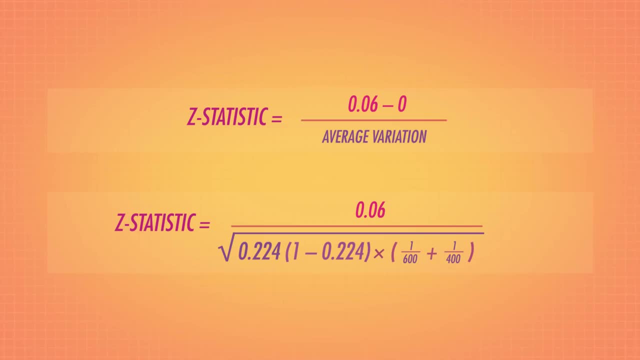 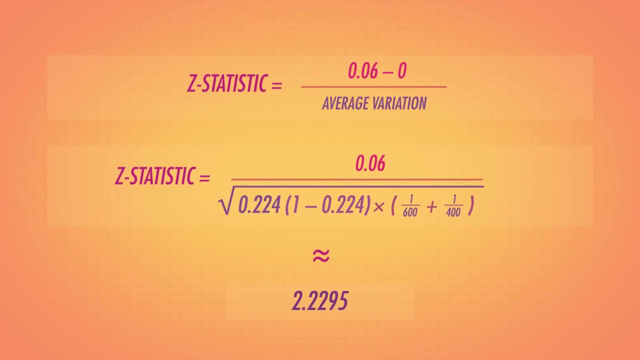 significant. We found evidence suggesting the null might not be accurate. There are two main ways of telling whether this z-statistic, which is about 2.2295 in our case, represents a statistically significant result. The first way is to calculate a critical value. 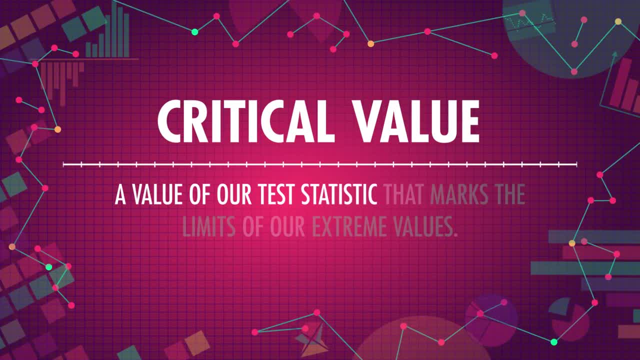 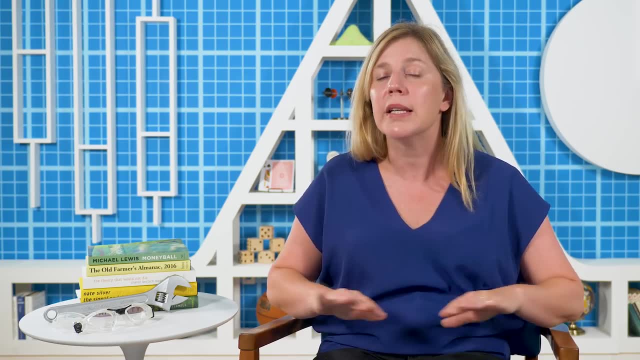 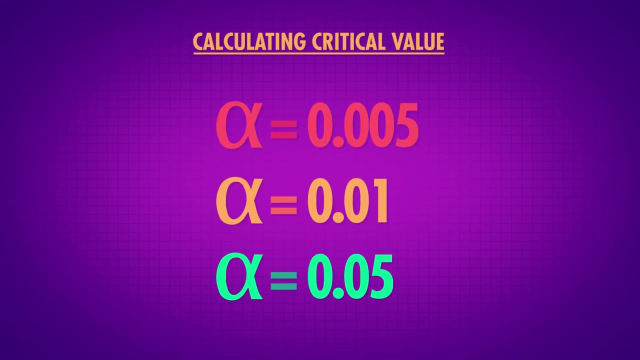 A critical value is a value of our test statistic that marks the limits of our extreme values. A test statistic that is more extreme than these critical values- that is, it's towards the tails- causes us to reject the null. We calculate our critical value by finding out which test statistic value corresponds. 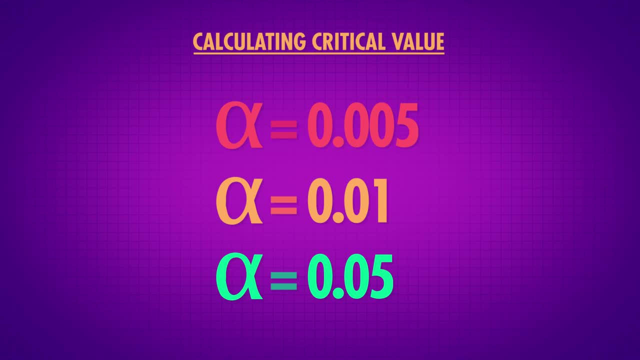 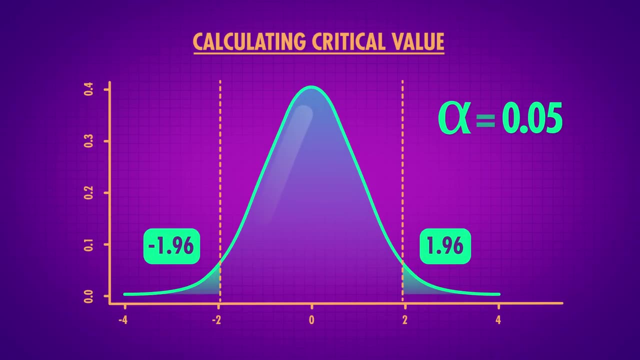 to the top 0.5,, 1, or 5%. most extreme values For a z-test with alpha equals 0.05, the critical values are 1.96.. If your z-statistic is more extreme than the critical value, you call it statistically. 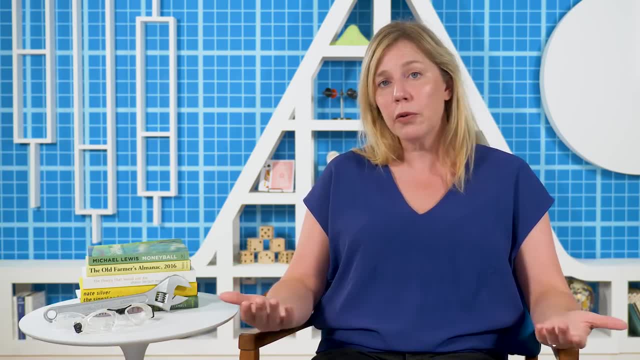 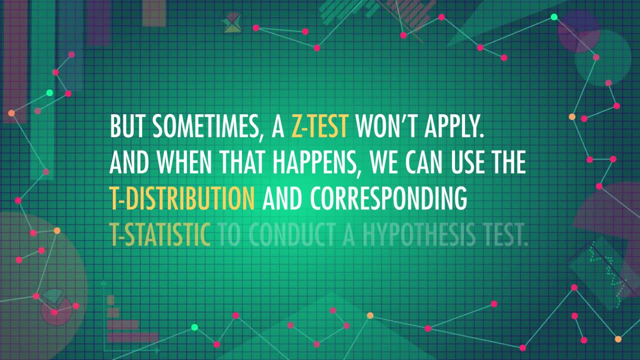 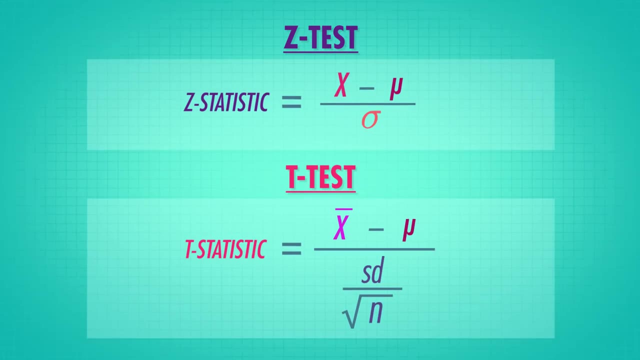 significant. So we found evidence in this case that the flu shot's working. But sometimes a z-test won't apply And when that happens we can use the t-distribution and corresponding t-statistic to conduct a hypothesis test. The t-test is just like our z-test. it uses the same general formula for its t-statistic. 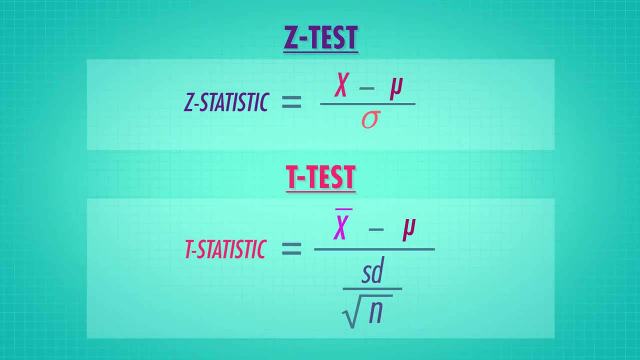 But we use a t-test if we don't know the true population standard deviation. As you can see, the t-statistic is the same as our z-test. We can see it looks like our z-statistic, except that we're using our sample standard. 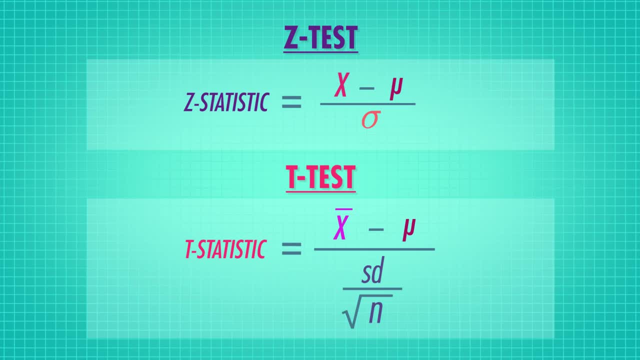 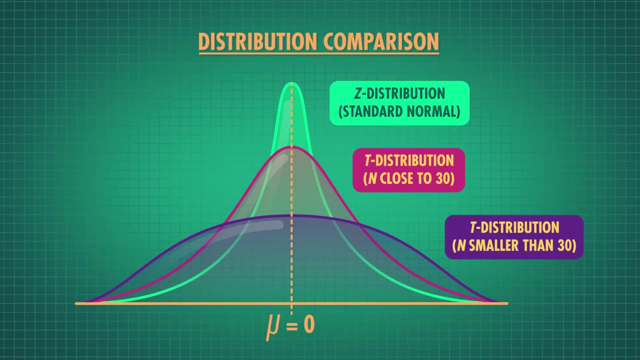 deviation instead of the population standard deviation. in the denominator, The t-distribution looks like the z-distribution, but with thicker tails. The tails are thicker because we're estimating the true population standard deviation. Estimation adds a little more uncertainty, which means thicker tails, since extreme values 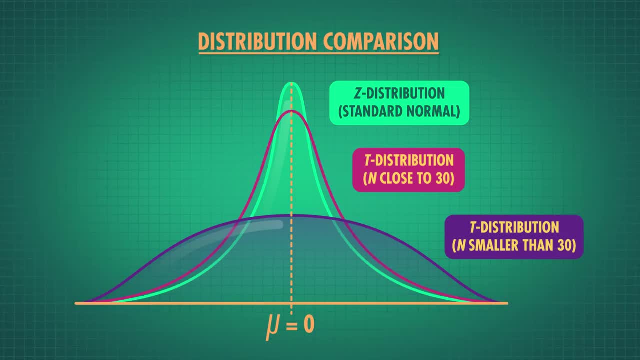 are a little more common. But as we get more and more data, the t-distribution converges to the z-distribution. So with really large samples we can get a z-stat, So we can get a z-stat. So we can get a z-stat. 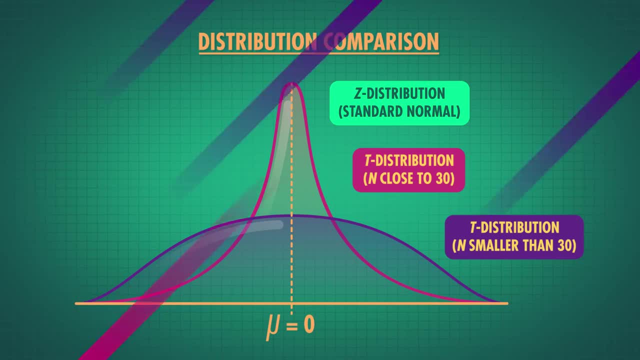 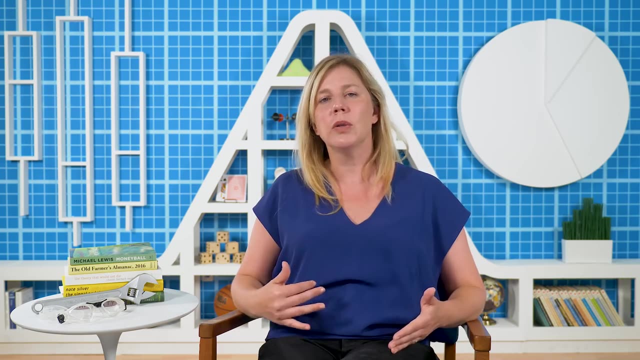 For examples, the z and t-test should give us similar p values. If we're ever in a situation where we had the population standard deviation, a z-test is the way to go, but a t-test is useful when we don't have that information. 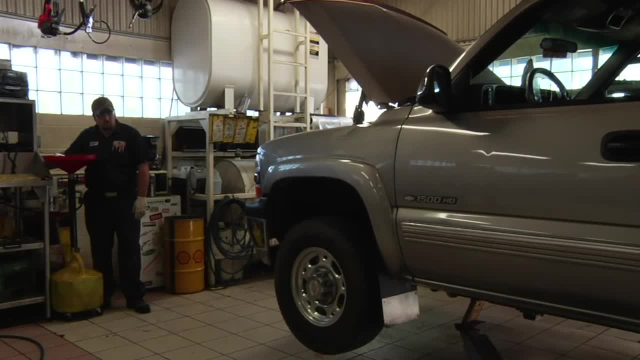 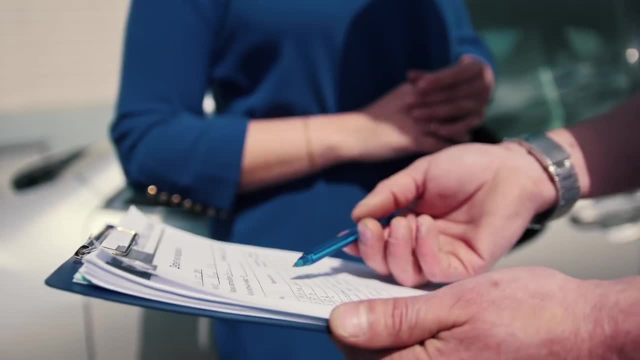 For example, we can use a t-test to ask whether the average wait time at a car repair shop across the street is different from the time you'll wait at a larger shop 10 minutes away. We collect data from 50 customers who need to take their cars in for major repairs. 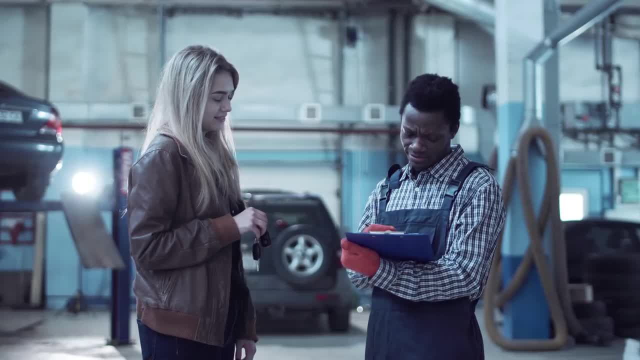 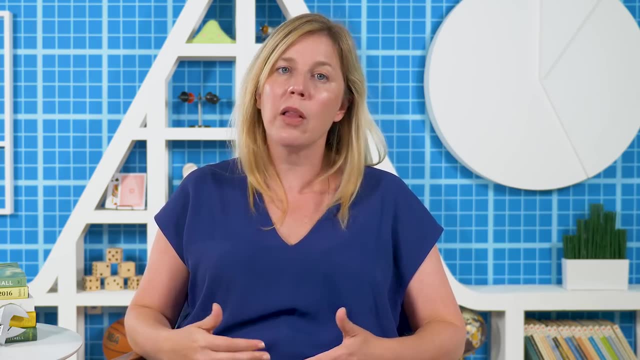 25 are randomly assigned to the smaller scale smaller repair shop and the other 25 are sent to the larger shop. After measuring the amount of time it took for repairs to be completed, we find that people who went to the smaller shop had an average wait time of 14 days. 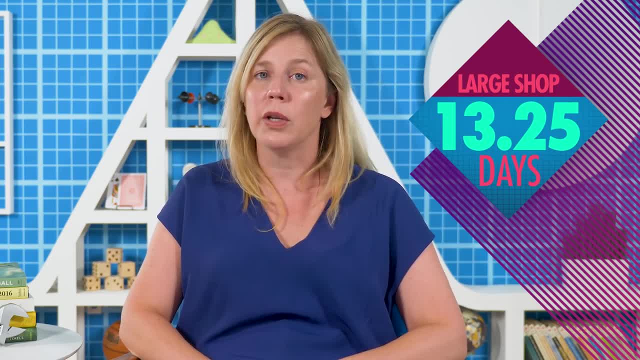 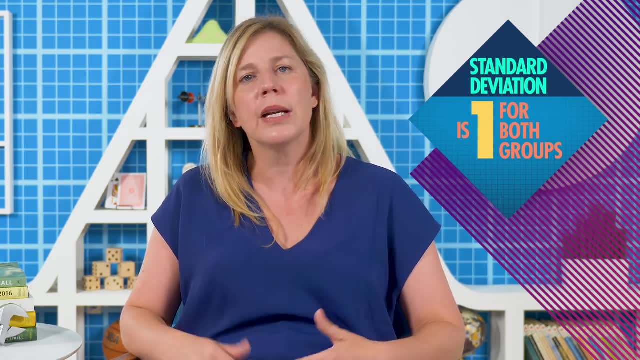 People who went to the larger shop had an average wait time of 13.25 days, which means there was a difference of .75 days in wait time. But we don't know whether it's likely that this .75 day difference is just due to. 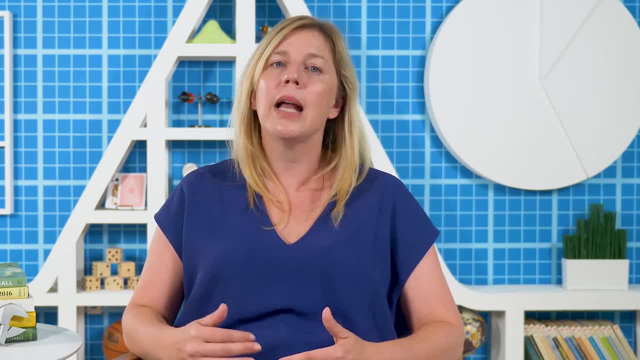 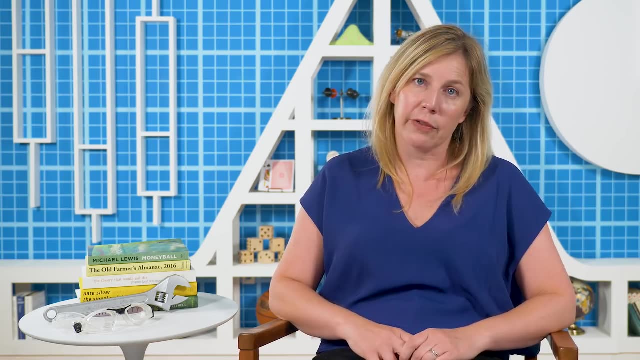 random variation between customers, At least not until we conduct a t-test on the difference between the means of the two groups. Before we do our test, we need to decide on an alpha level. We set our alpha at .01 because we want to be a bit more cautious about rejecting the 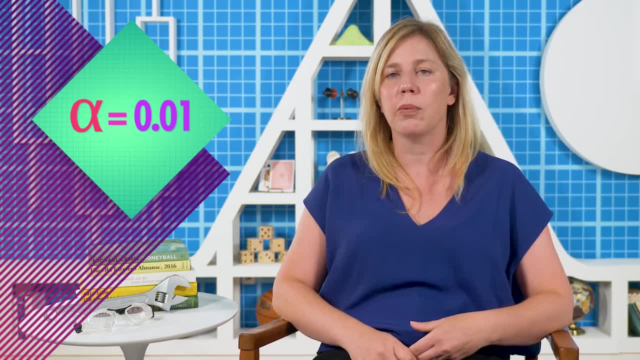 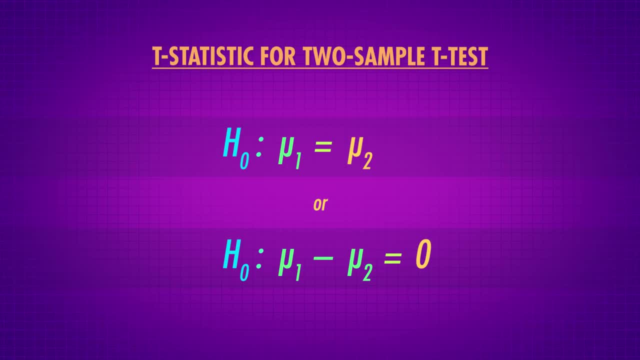 null hypothesis than we would be if we used the standard of .05.. Now we can calculate the t-statistic for our two-sample t-test. If the null hypothesis was true, there'd be no real difference between the mean wait times of the two groups. 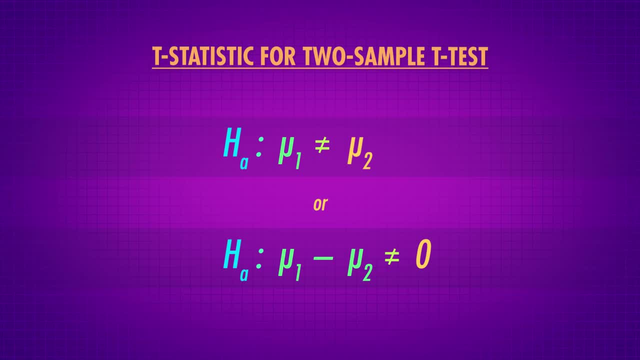 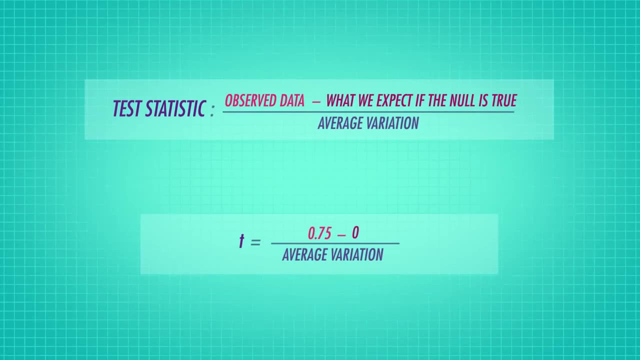 And the alternative hypothesis Is that the two means are not equal. The two-sample t-statistic again follows the general form. We observed a .75 day difference in wait times between the groups. We'd expect to see a difference of zero if the null were true. 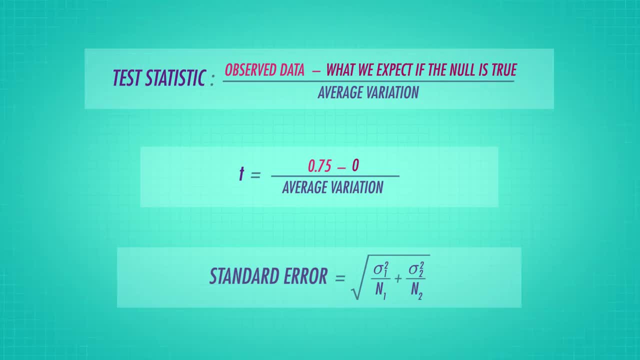 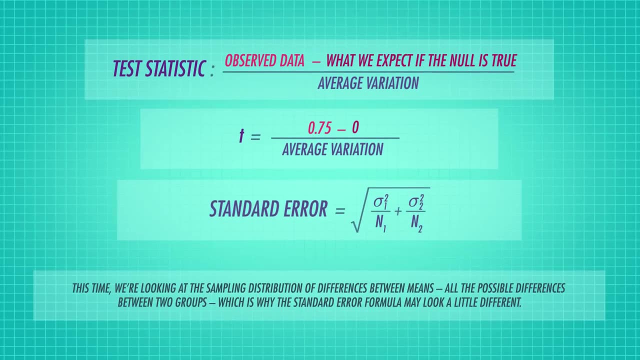 Our measure of average variation. here is the standard error. The standard error is the typical distance that a sample mean will be from the population mean. This time we're looking at the sampling distribution of differences between means, All the possible differences. This is why the standard error formula may look a little different. 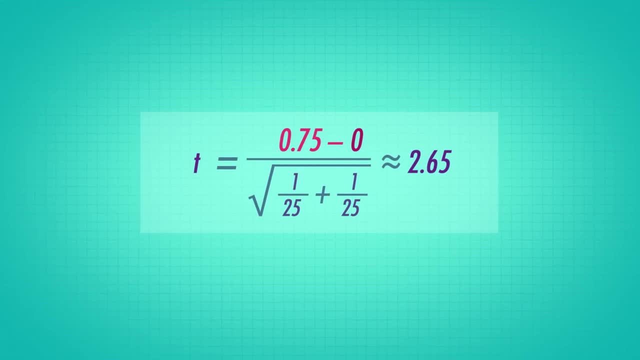 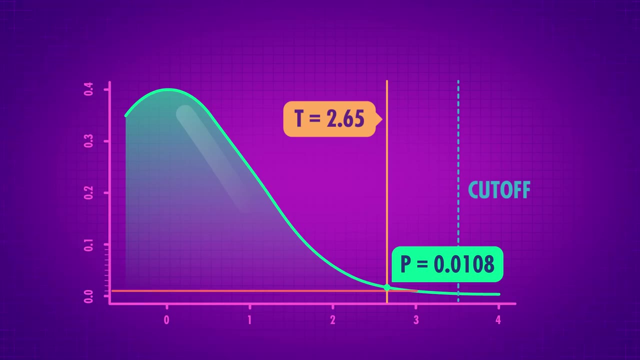 Putting it all together, we get a t-statistic of about 2.65.. If we plug that into our computer, we can see that this test statistic has a p-value of about .0108.. Since we set our alpha at .01, a p-value needs to be smaller than .01 to reject the null. 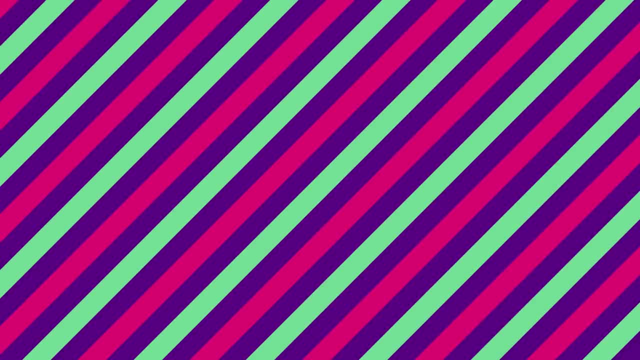 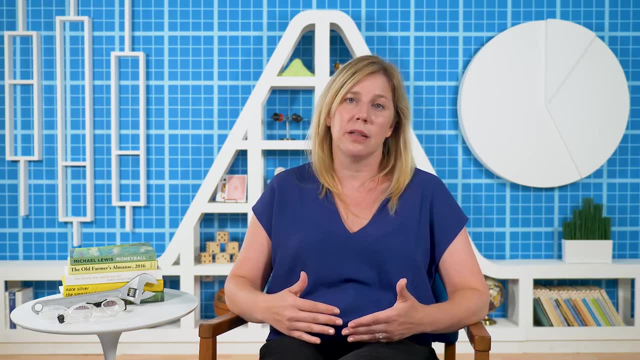 hypothesis. Ours isn't Barely, But it isn't So. it might have seemed like the larger repair shop was definitely going to be faster, but it's actually not so clear, And this doesn't mean that there isn't a difference. 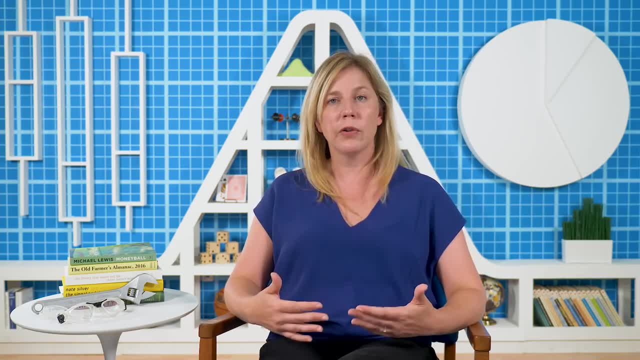 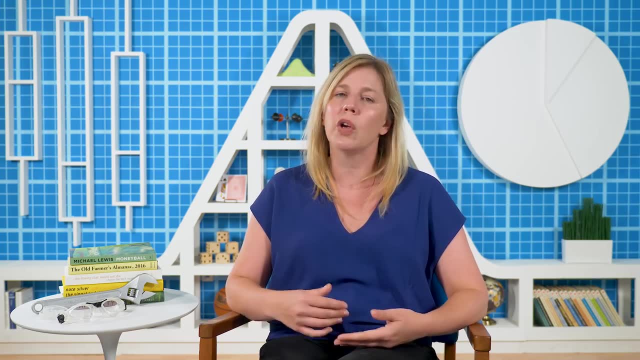 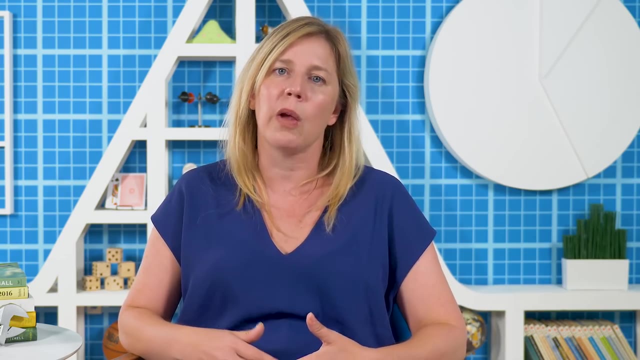 We just couldn't find any evidence that there was one. So if you're trying to decide which shop to take your car to, maybe consider something other than speed- And we could do similar experiments for cost or reliability or friendliness- You might notice that throughout the examples in this episode, we used two methods of deciding. 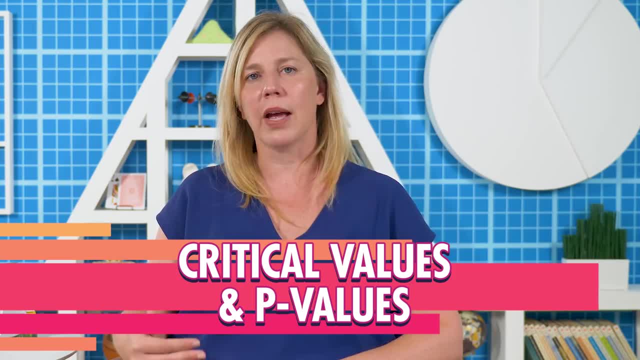 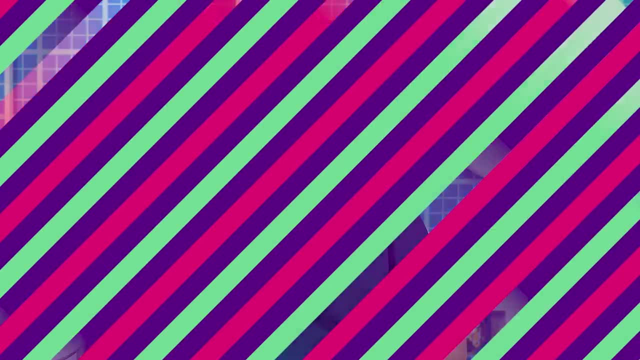 whether something was significant. Critical values and p-values: These two methods are equivalent: Large test statistics and small p-values. both refer to samples that are extreme. A test statistic that's bigger than our critical value would allow us to reject the null hypothesis.